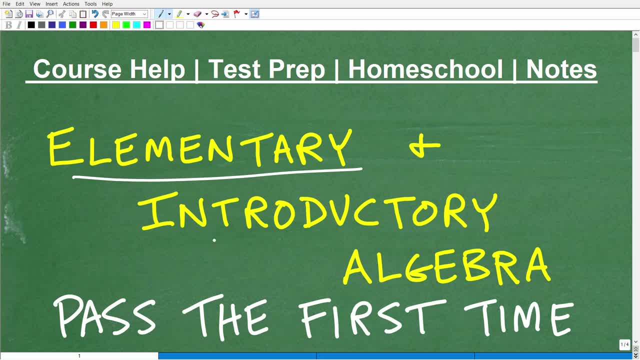 Okay, let's talk about elementary algebra and introductory algebra, And the whole point of this video is to give you some tips so you can pass these courses the first time. So oftentimes people take elementary algebra or introductory algebra at the college level, and it's generally adults going back to school. 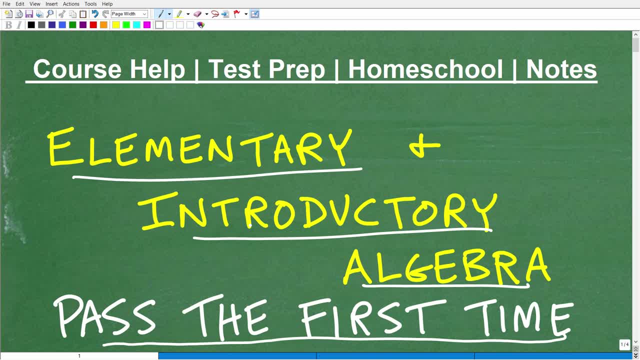 This is the kind of most typical type of student that takes these courses. So maybe you've been out of school for several years and you're going to have to take some basic algebra course, which is pretty typical. again that it's referred to as elementary algebra or introductory algebra. 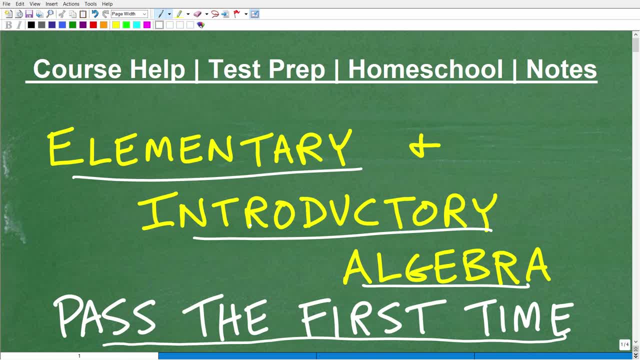 or some other type of basic algebra. They're effectively the same course, but I'm going to give you some tips that you need to kind of pay attention to. So when you take this course, if you've been out of school for several years, you actually pass it the first time. 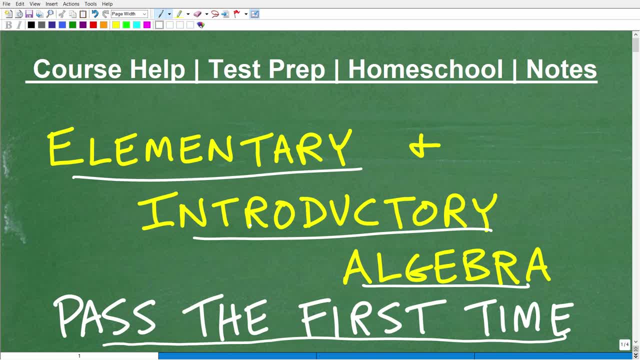 So you want to be kind of mentally prepared to go back to school and take these courses. So if you stick around for a couple minutes, I'm going to give you some good things that if you follow my guidance, my tips, that you will be successful and pass these courses. 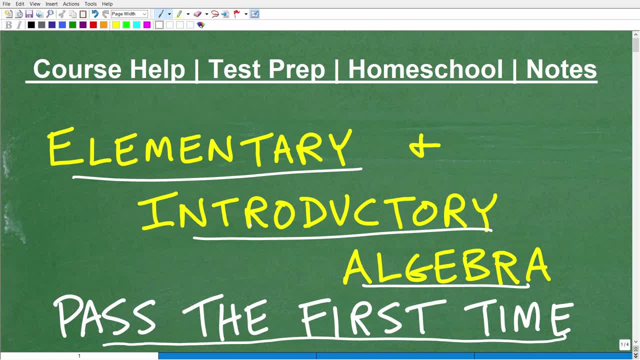 But before we get going, let me first quickly introduce myself. My name is John. I'm the founder of Tablet Class Math. I'm also a middle and high school math teacher. I'm going to leave a link to my math help program in the description of this video. 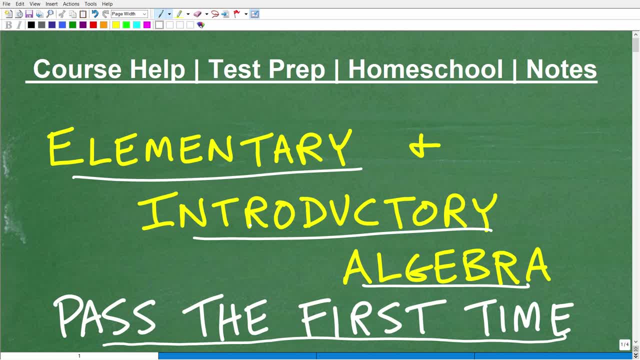 But I like to think of myself as someone who explains math. Of course I'm a teacher, but I really like to explain math And very clear and understandable terms so anyone and everyone can learn this stuff. So if you're at the middle school, high school or college level, 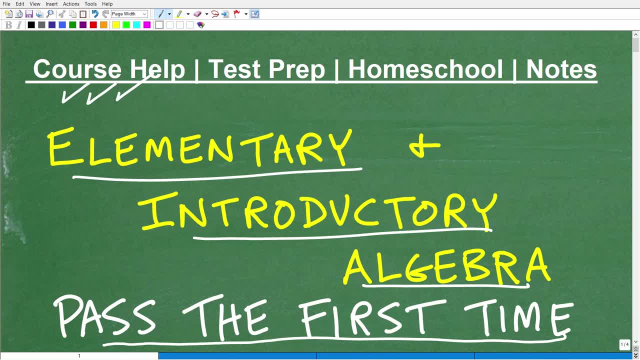 I can definitely help you get through your respective math courses Now. if you happen to be preparing for any sort of test that has a math section on it- and there's a lot of them out there- I'm talking about things like the GED, SAT, ACT, GRE, GMAT, ASVAB. 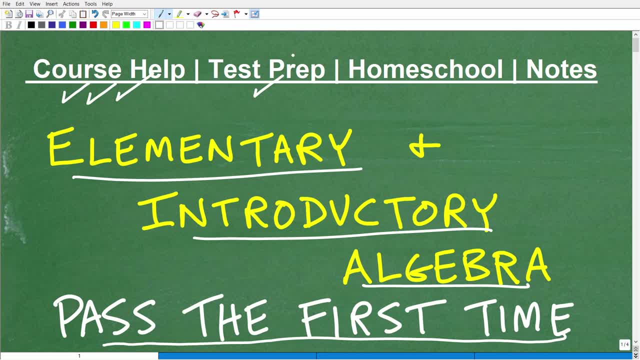 ACUPLACE or CLEP exam, maybe a teacher certification exam. I can definitely help you prepare and pass those exams. If you homeschool, you've got to check out my homeschool math courses. I was just recently voted number one for middle school and high school mathematics by a major homeschool publication. 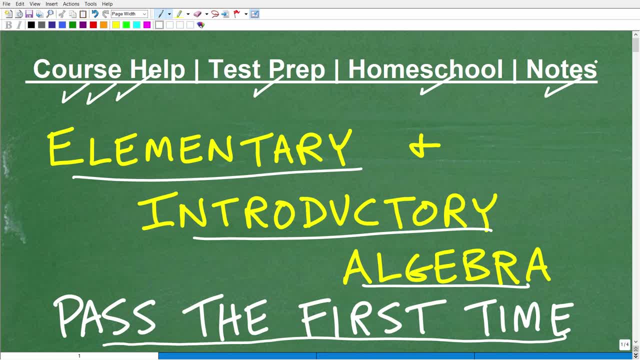 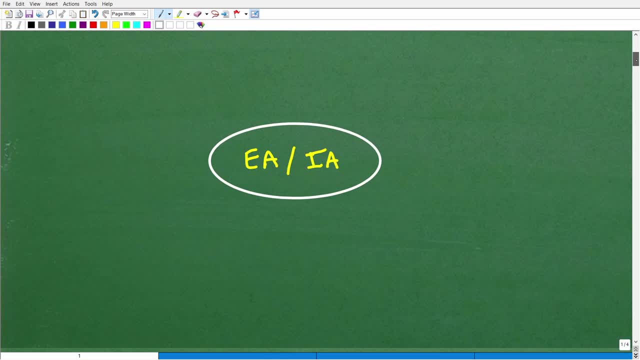 Pretty excited about that, And if you need some math notes, I'm going to leave links to my math notes in the description of this video. Okay, so let's get into it Again. this is just going to be some general guidance on those of you out there that are going to be taking elementary algebra or 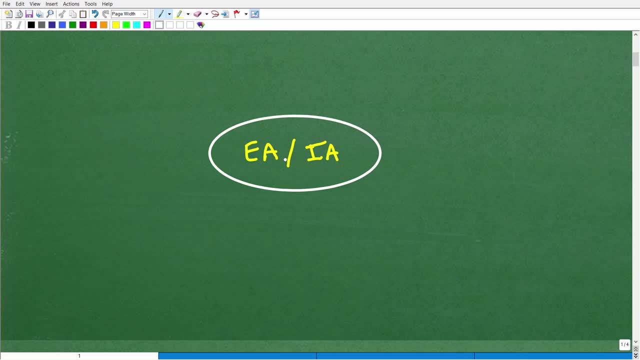 introductory algebra or some sort of basic algebra. And again, these are course descriptions that are generally at the community college level. okay, So the first thing is, if you're thinking back to your high school years, you're like, well, what, what am I going to be expecting? 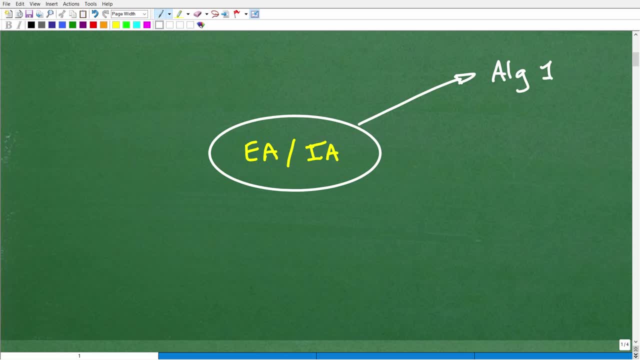 Well, this is effectively, for the most part, equivalent to high school algebra one. Okay. so, if you can remember back- and typically most students took this as a freshman- there's also going to be some aspect of maybe like pre-algebra, which is like a 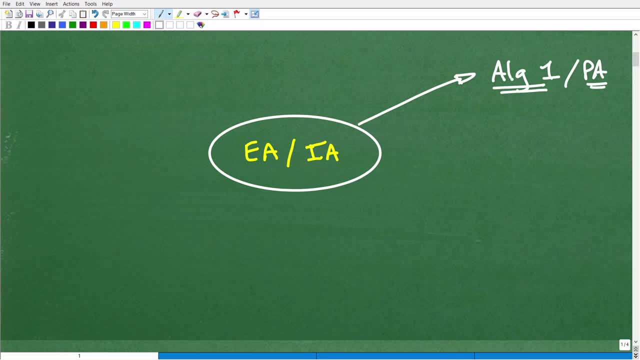 typically an eighth grade course. So we're talking eighth, ninth grade level mathematics. Okay, Now, with that being said, there is a lot to be covered in high school algebra one. So this is a full one-year course and these courses here. 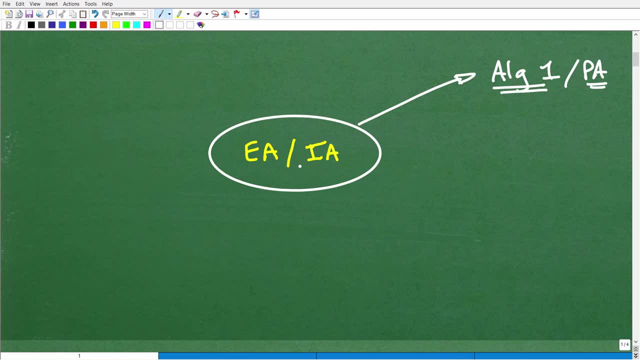 depending on your college, sometimes could be like one semester course courses. So the one thing you need to be mindful is you had. you know I'm speaking in generalities because every college is going to be a little bit different, but in this course here, 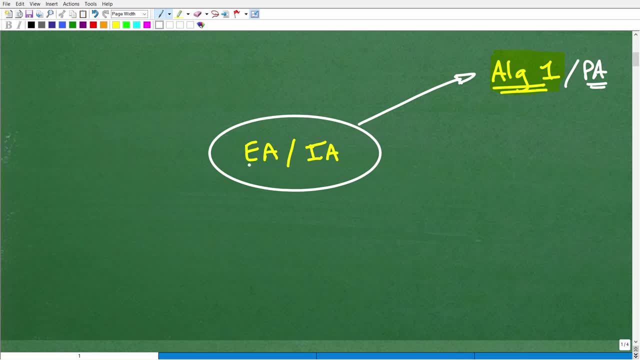 students, high school students- get one year, and oftentimes these courses are going to be, like you know, one semester, excuse me. So that means the pace is going to be a lot faster. So that's the first thing I want you to kind of know is that the pace is going to be generally quick. 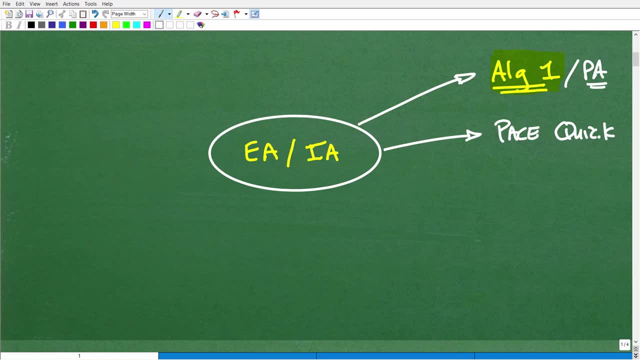 Okay, so you're going to have to be ready to. you know, you know, right, when the course starts to be prepared for a faster pace. Now again, there's exceptions to this, but generally speaking, this is how it kind of works at the college level. So. 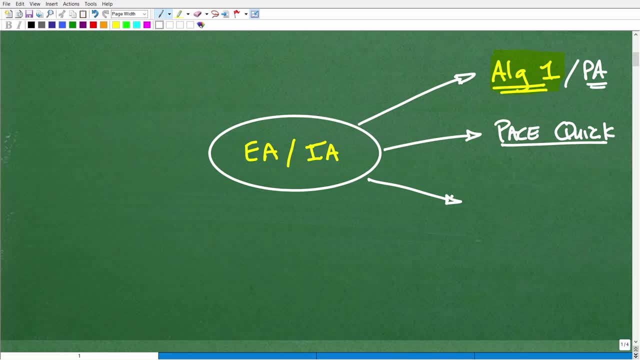 with that being said, you're saying: well, you know, I didn't do well in high school mathematics. I'm very concerned about this. I want you to know- and this is more directed towards those of you that are adult learners- 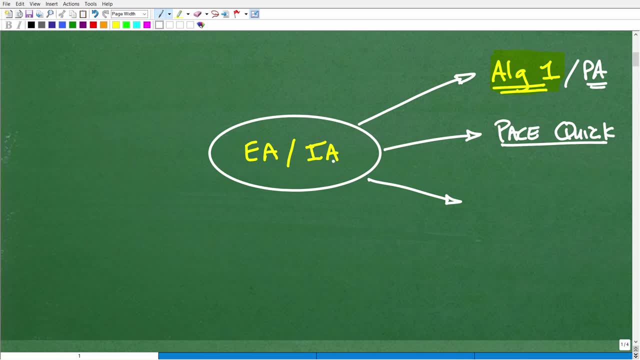 because, again, elementary algebra and introductory algebra are typically, you know, course descriptions of college level courses And I would say, the majority of people that are taking these courses are people going back to school. But even if you're 18 and you didn't do well in high school mathematics, you need to forget all that. 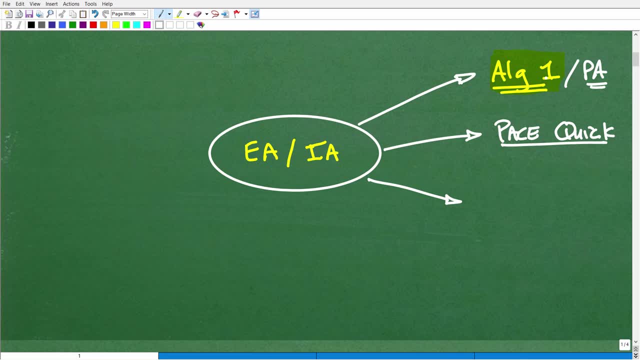 Okay. so in other words, if you didn't do well in high school or middle school and you're like I don't do well in math, forget all that. You are a different person. So, because you are an adult and you are choosing to go to school and learn and work, 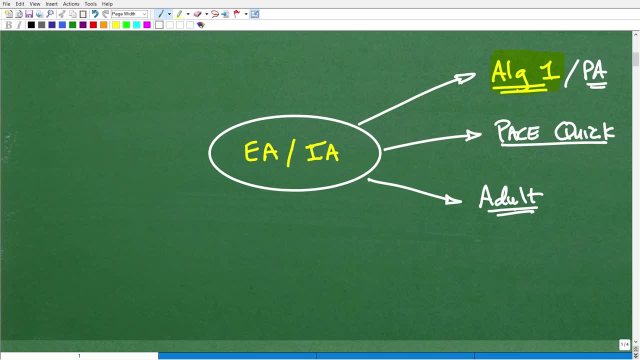 towards a degree or a certification. you know you're committed to a big goal in your life. You're not the same as a young- you know- 14,, 15 year old high school student that is distracted by their friends in the classroom. 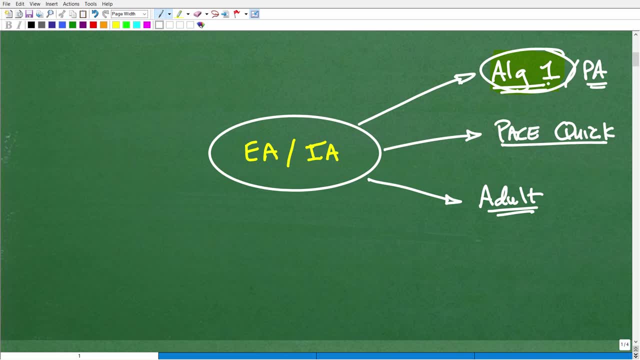 You're a different person. So these students here, they can do well in math, But they're you know. of course, even myself, way back in the good old 1980s, I was completely distracted. I wasn't a great student. I was talking to my buddies and doing all kinds of stuff, but of course, 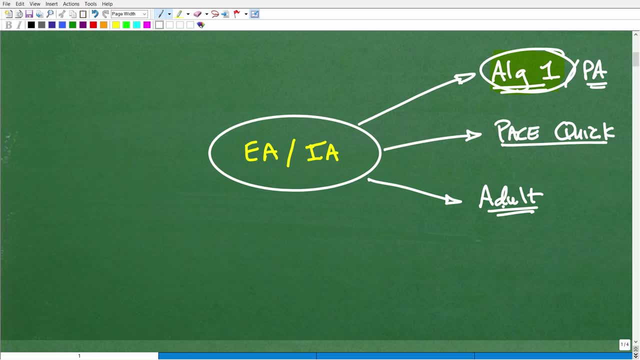 when you go to college you're much more responsible and committed, so you need to give yourself kind of a mental reset that as an adult you're going to be a much better learner than you were in high school. so your track record back then really is to go. don't. don't bring that towards what your your potential. 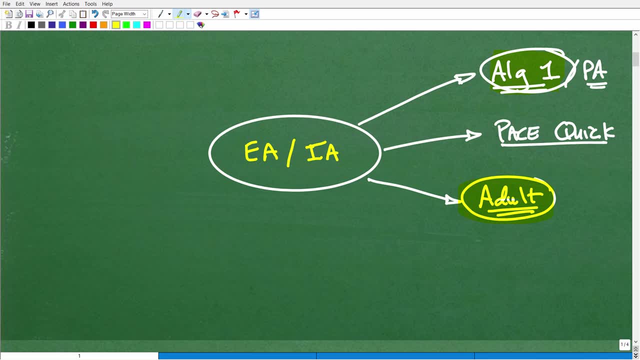 or your capabilities are as an adult. I'm here to tell you that you can do very well in mathematics. of course, you know, if you're still, you know, just you know- find yourself distracted and things like that, of course that's gonna be an issue, but that's not going to be the case at you know, at a college level type. 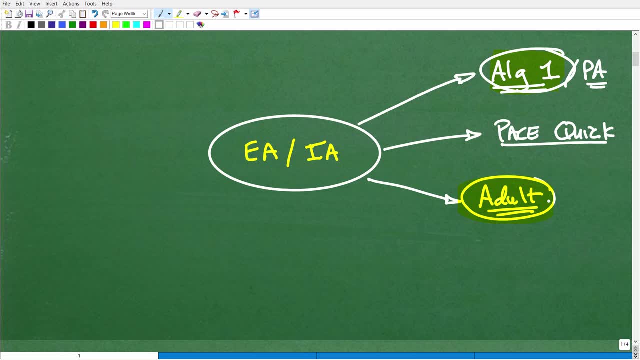 of course. so, as an adult, okay, you're going to have the kind of the soft skills to be successful. and what are those things? well, you know commitment, dedication, all those different types of things. so you're gonna have to be willing to put in the work. okay, if you're paying. 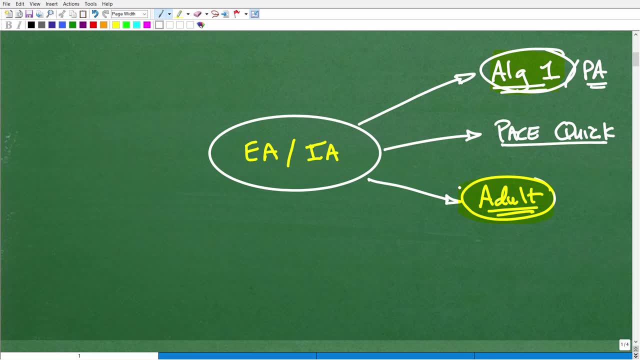 out-of-pocket for a college course, then you know, you know you're obviously, you know, want to get your money's worth and pass this course. so let's talk about some things that are gonna be critical for you. so the first thing is you definitely need to learn how to take excellent math notes. okay, so that a lot. 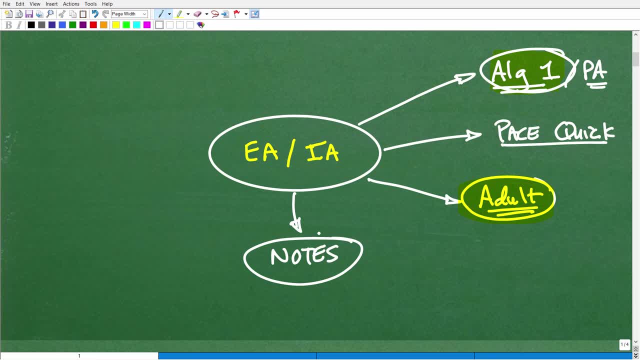 of information is gonna be coming at you, so if you don't like taking notes, you need to get to taking notes, because you're gonna have to take a lot of notes in this course, okay, so whatever the teachers writing down or presenting, make sure you're right and just get yourself a good old-fashioned third-ring binder with a. 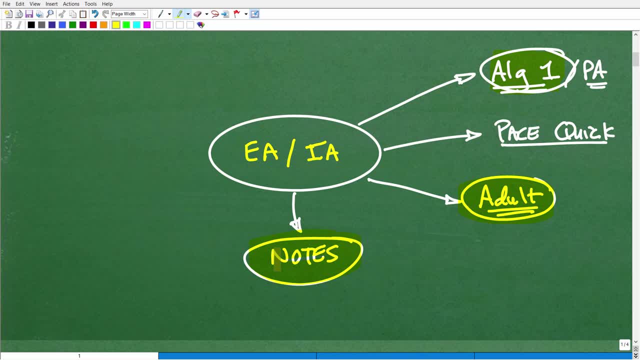 pencil. okay, so you should be taking a lot of notes. it's critical now, note taking. some of you might be like: well, they give me the information. there's unlike work. well, online worksheets, etc. I don't need to take notes because I can always download the information. the whole point of note-taking. 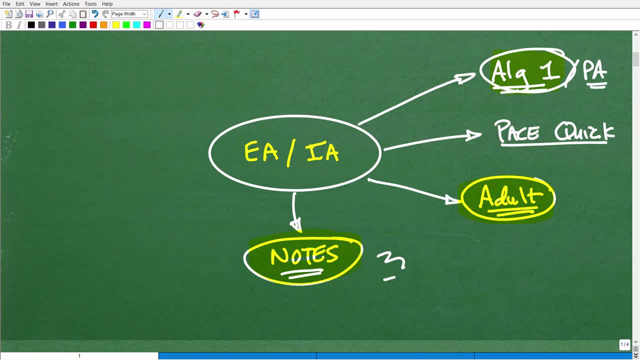 is your interaction. when you're writing things down and just like you know that that is, this activity goes to your focus. okay, focus is the key. you have to be tremendously focused. and when you're focused on the information writing that down, not only are your laser focused on the information. the teachers saying this. 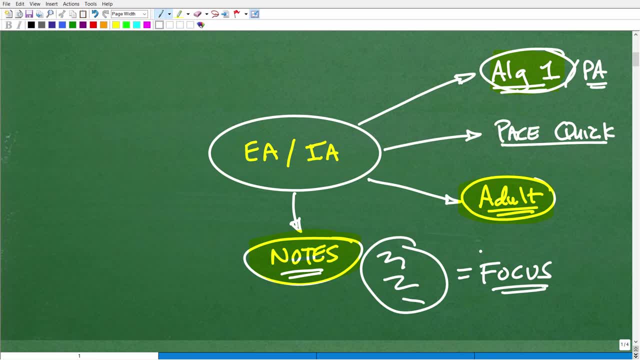 whole activity of you writing things down, this kinesthetic kind of learning process, is going to go towards your retention. okay, so you got to take notes, you got to review your notes. these are, like some of the basic, basic things, academic skills- that maybe you didn't you know. 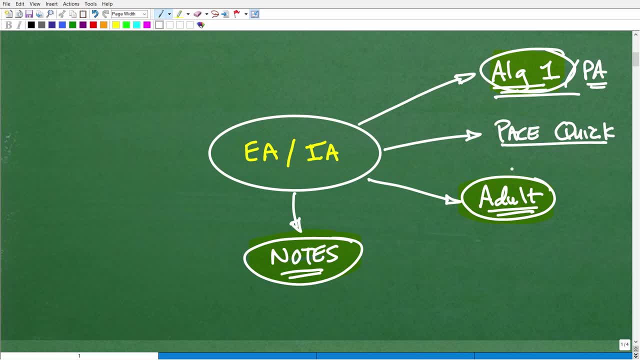 practice in high school, but you're gonna have to learn them, you know, as an adult in college okay. so excellent note-taking is, you know, critical okay- and I kind of like to say this on some of my other YouTube videos- is that, and I've seen this- 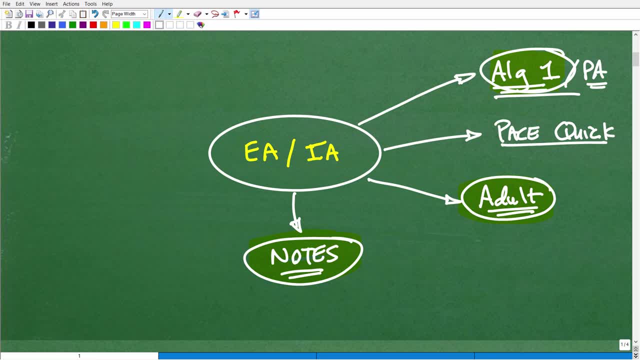 over decades of teaching mathematics, those students who take great notes almost always end up Getting the top grades, and the reverse is true. Those students who take poor notes or are like really not organized well and whatnot, those students generally end up with, you know, barely passing the course. if not, you know failing the course. So, anyways, be prepared to take great notes. 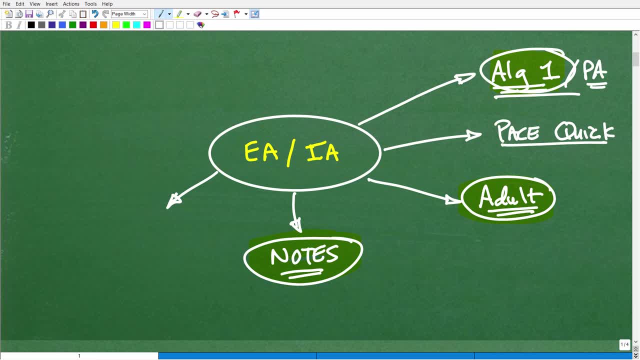 Okay, so now, another thing you can do is the following. I'm going to really recommend this is, if you know that you're going to be taking elementary algebra or introductory algebra, I'm going to suggest getting into some sort of program. Okay, now, what do I mean by that? I'm going to put this in parentheses and this might be kind of a shameless plug for my program, but you may want to consider starting to learn algebra before you take this course. 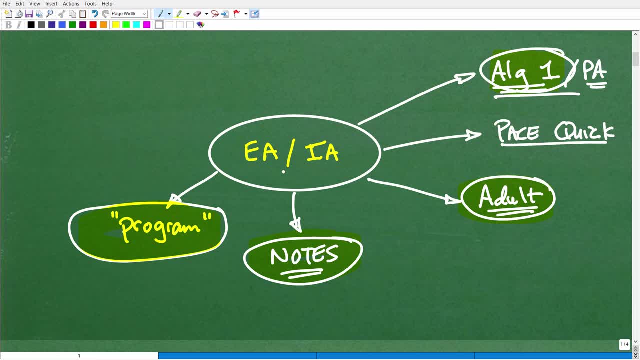 I'm going to strongly suggest that. So, if you know, oh, in a couple months I'm going to be taking this course and you have some, you know, anxiety about it. If you take one of my courses, like my introductory algebra or pre-algebra algebra- one course- you're going to get ahead, Okay, you're going to build momentum, you're going to learn skills, which is going to make things a lot easier for you when you actually take this course. 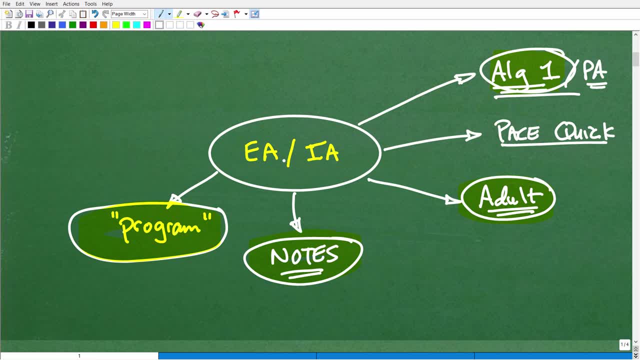 Remember, the topic of this video is to get you to pass these courses the first time. So if you get an excellent program where there's a lot of great instruction, It's like my YouTube channel. I have a lot of different videos, but it's not organized in a specific kind of curriculum. 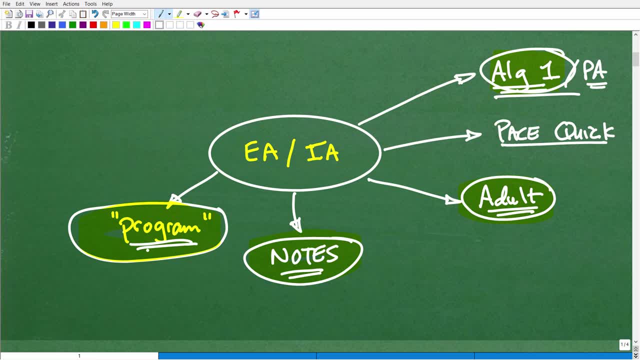 So if, for example, if you take my course, okay and you're not going to complete the course because that takes a long time, but if you start learning the material, it's going to really help build momentum for you in this course. 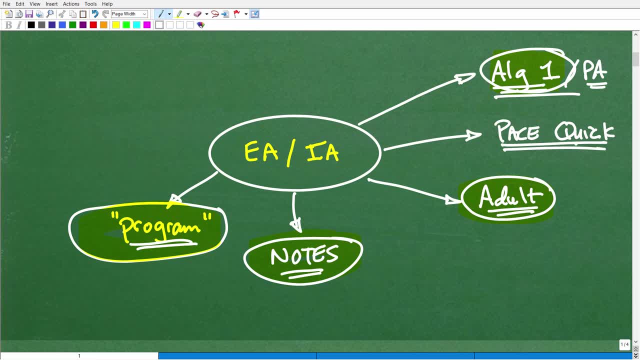 Because, remember, this material is going to be coming at you a lot faster. Plus, having a program like my, something like what I have, is a kind of a nice supplemental course, You know, a program to help you when you don't understand from your teacher, oftentimes too, because- let me just say this much- sometimes you're not going to be taking this in a classroom. 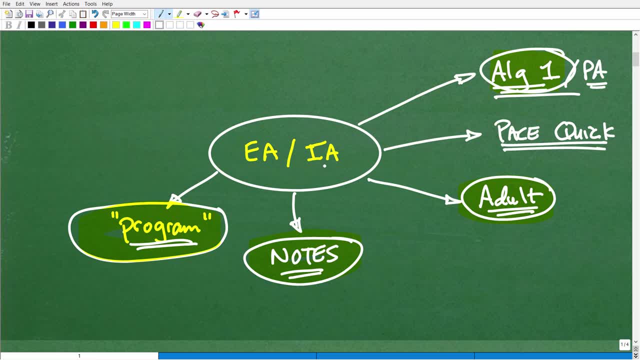 Sometimes you might be taking this online and I hate to say it, but a lot of the programs that I've seen online that colleges offer with these courses are not the best quality. They're quite confusing and a lot of students struggle. So not only is the instruction coming at students a little bit differently, they also got to deal with a 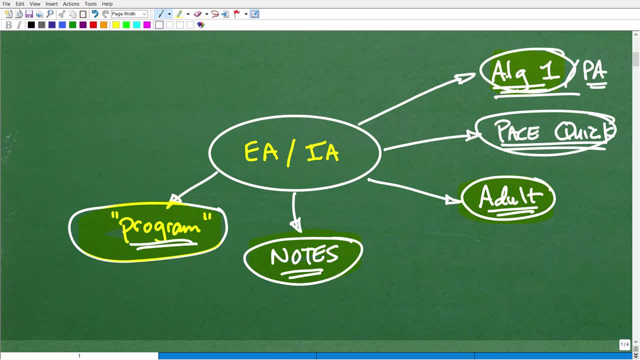 a fast pace and they're also going to deal with not maybe practicing all these great academic habits for a long time. So that can lead to a bad, you know- outcome. ie not passing the course, All right. so another thing that you have to kind of really be ready- and I'm kind of maybe you know some of this stuff kind of overlaps here- is that you have to be kind of mentally ready to work. 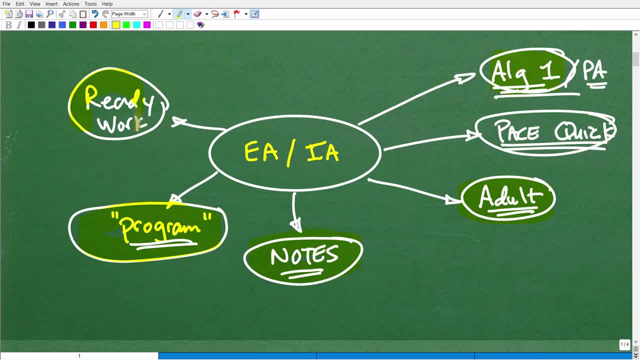 Okay. In other words, there's no shortcuts. and if you're not prepared 100% to be committed to this- I'm talking about being immersive, doing all the homework you know, not skipping any classes. I mean, you have to be ready to work and not fall behind. 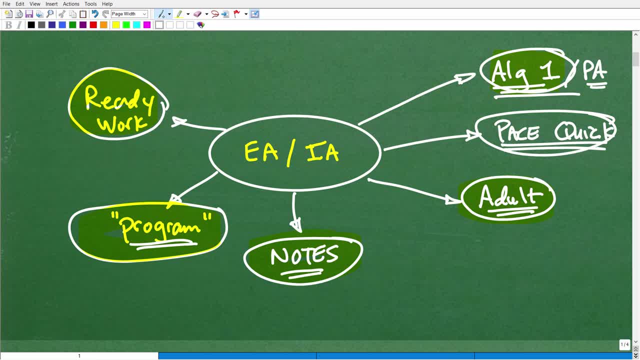 Okay. So if you're taking this, you're like, and you're just, maybe your your level of commitment is not quite there, or maybe you have a lot of distractions going on in your life. You might want to think about postponiness, but I'm here to tell you there's not going to be any shortcuts. 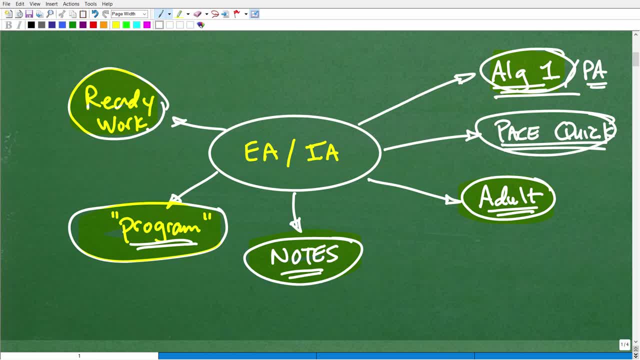 Okay, So you're going to have to put in the work to do the right things. You know again, if someone out there is saying, no, you don't have to do that or it's not so easy, Well, guess what. 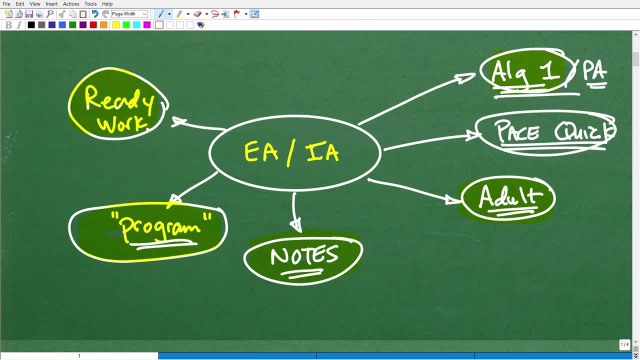 That's bad advice, and nothing good comes easy. So be ready to work. Okay, Have that kind of you know carved out in your calendar, especially if you have some anxiety about you know mathematics. Okay, So put in extra time. 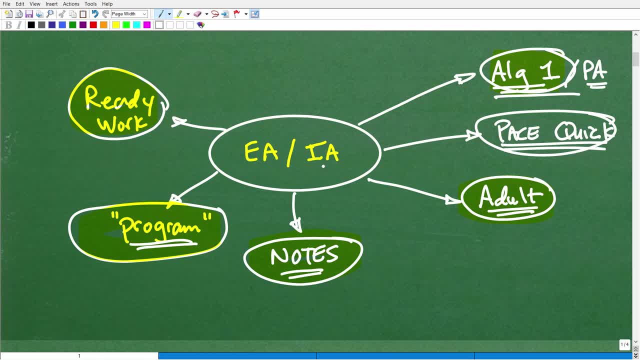 All right. So whatever you think you need to learn, maybe double the Amount of time And a course like this you're going to have to put in a minimum of an hour, maybe an hour to two per day, And even on the weekends, because this course is generally going to go pretty quick. 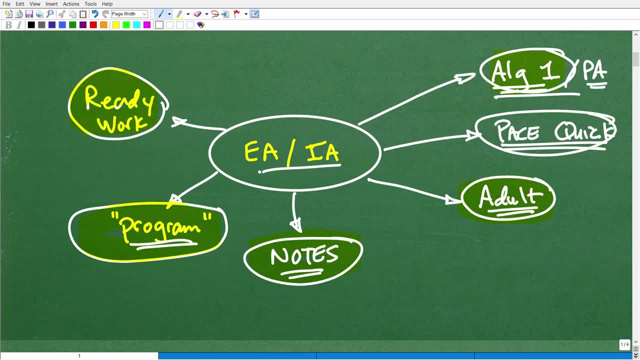 Okay, Again, I'm speaking to those courses that are going to be one semester. Okay, So the last tip I'm going to talk about here is to talk to your teacher. Okay, Ask questions. Be that pesky student That is saying: you know. hey, teacher, I need help. 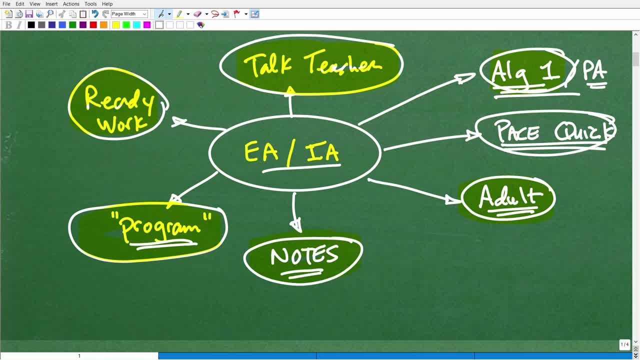 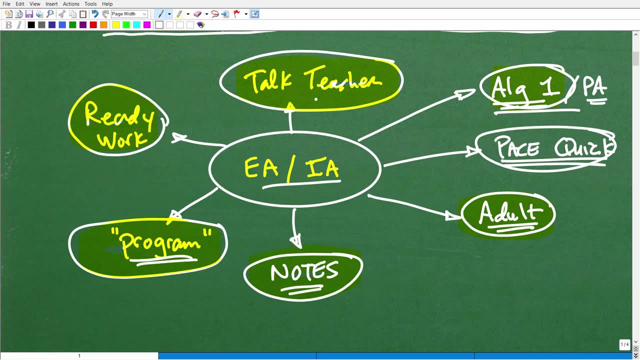 You know I'm falling behind. I don't understand this. Ask questions, Be demanding, Because this is going to show your teacher a couple things. One: you're going to get the teacher answering questions Now, even if you don't understand everything they're talking about you. can you know, maybe use a program like mine to learn? 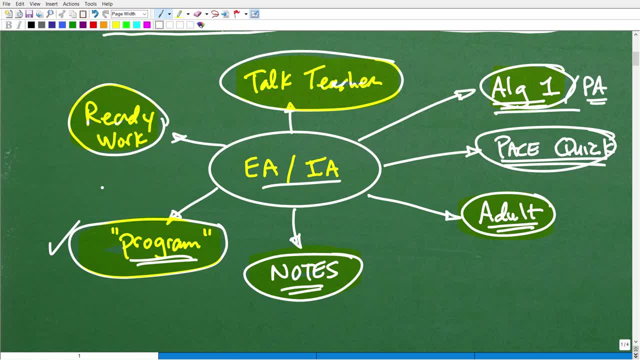 When you're engaged with your teacher, okay, your professor, whoever the case might be, it's showing them, okay, that you care, that you're engaged, that you're like. you know this person wants to pass this course. 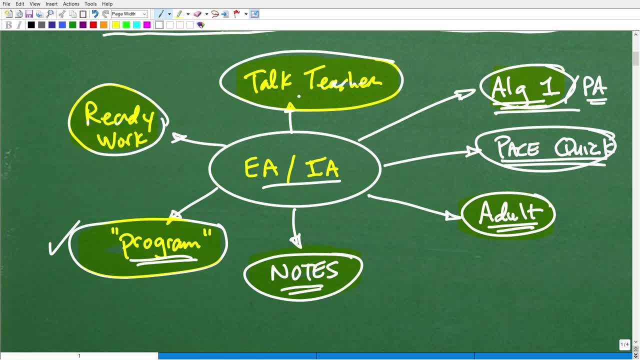 It's really, really important. So if you are falling behind, let's say you take a test and you get 77%, that is not good. Okay, Even though you passed, you need to be hey teacher. what did I do wrong? 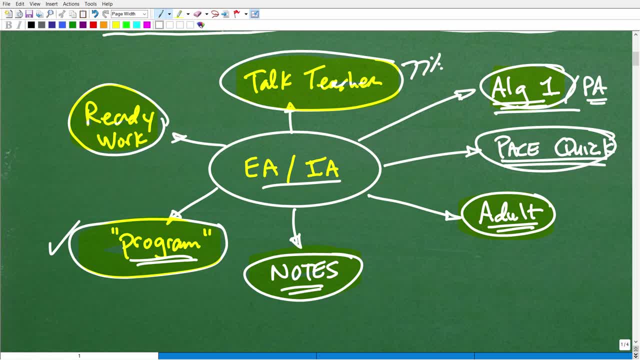 What can I do better? Can I make up any points here? So you have to be highly engaged with your teacher. You don't want to be a passive student. Now I'm going to tell you right now this also. it's kind of an unwritten rule. 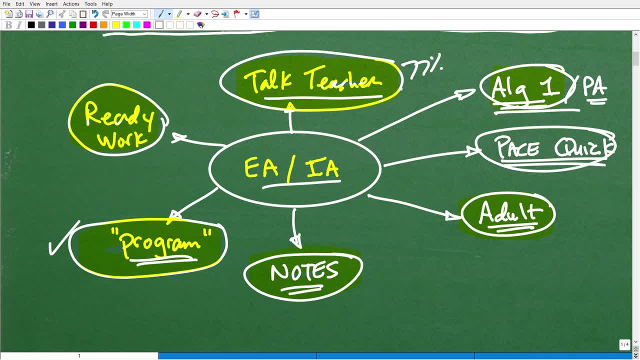 Teachers aren't going to tell you. It's been, I've been a teacher and I'm going to tell you right now that teachers can find points. You're like: what are you talking about? Well, believe me, if a student gets a 69.2% and they need a 70% to pass, and that is it, that was their final grade. 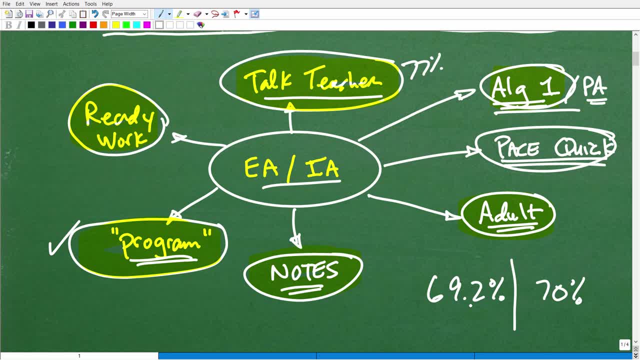 but this particular student was just a hard worker, engaged and whatnot. believe me, that teacher can just pull some points from the universe and get that person over to 70%, okay. However, the reverse is true. If the teacher thinks that you're not really engaged, you didn't put in the work, you weren't really trying. 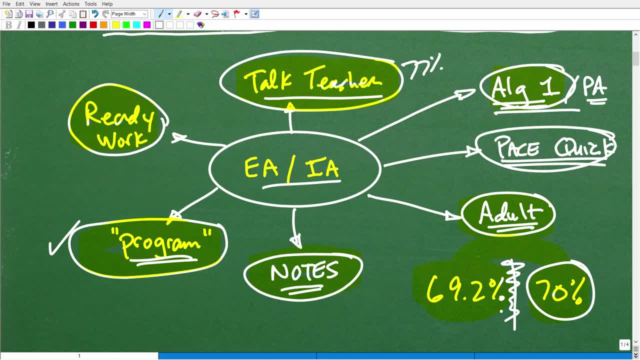 then you know there is that kind of like gray area that a lot of teachers aren't going to. you know kind of reward you So make sure you are engaged, you're asking questions, but if you follow all of these kind of you know guidelines here, 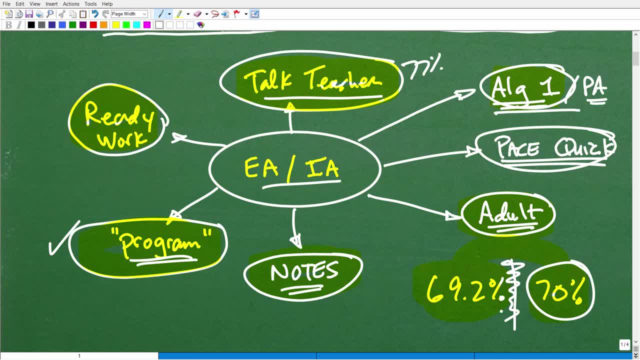 you know you will pass. okay, Definitely you will pass. And of course you know this is elementary algebra, introductory algebra, and that's typically not going to be enough in terms of your minimum requirement for college or whatnot.